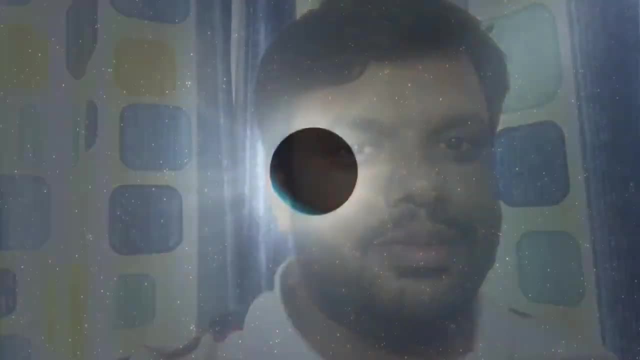 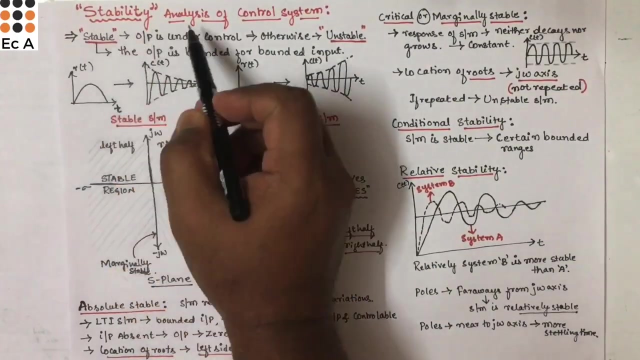 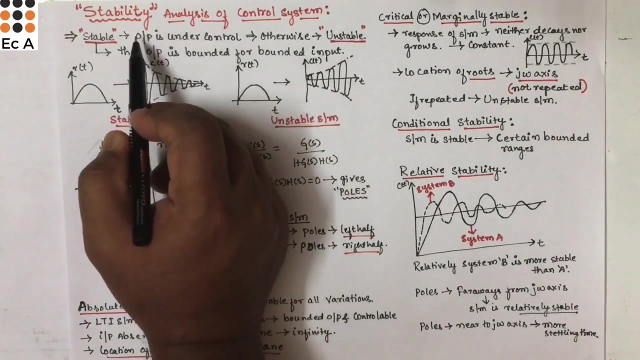 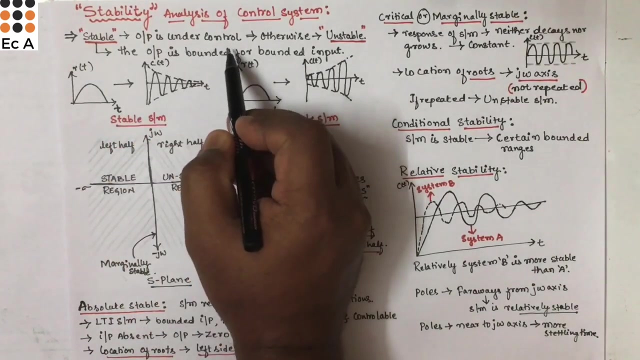 Hello friends, welcome to EC Academy. In this lecture let us understand the introduction to stability analysis of control system. After transient response and steady state, error stability is very important factor of any control system. A system is said to be stable if the output is under control. 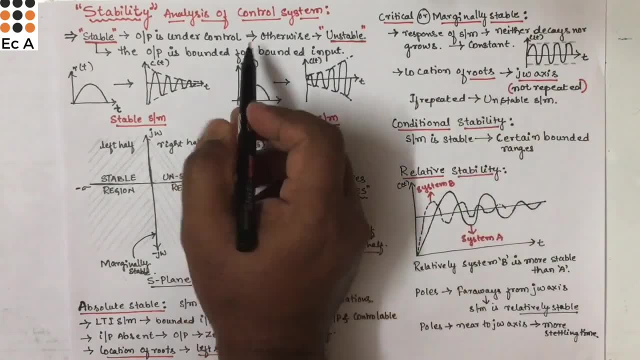 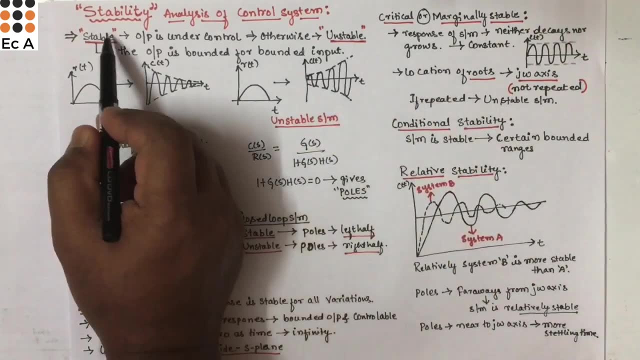 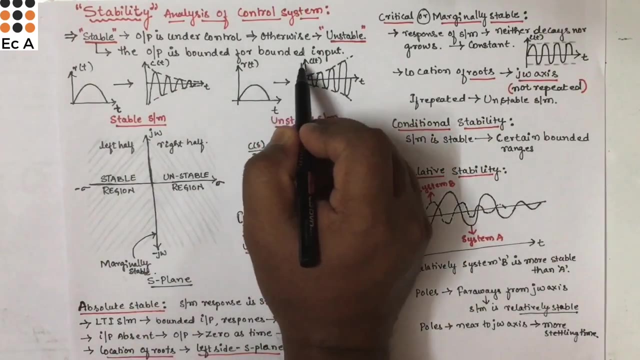 Otherwise the system is unstable. So if the output of the system is not under control, we will call such type of system as unstable system. In a stable system the output is bounded for bounded input. So we can say: in a stable system, if input is bounded, output will be bounded. 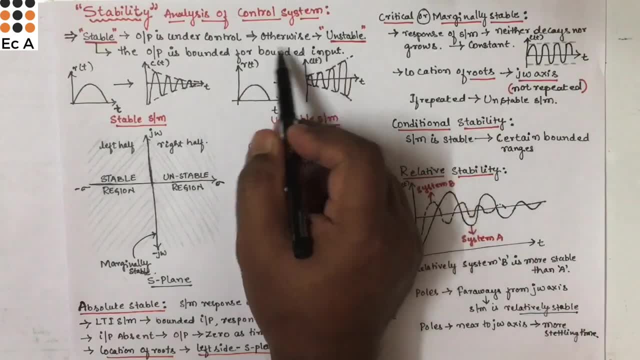 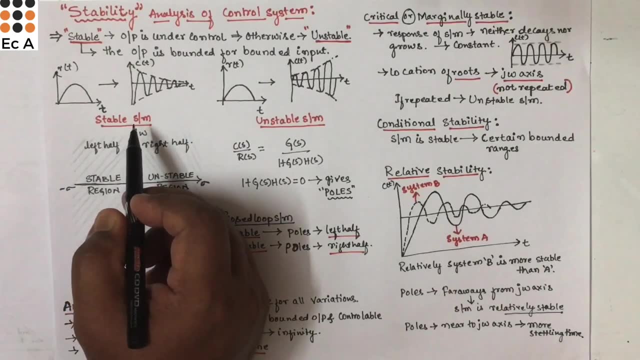 So we can say: in a stable system, for a bounded input we will get a bounded output. A system is said to be stable if the transient response vanishes as the time approaches To infinity. So you can see this figure. 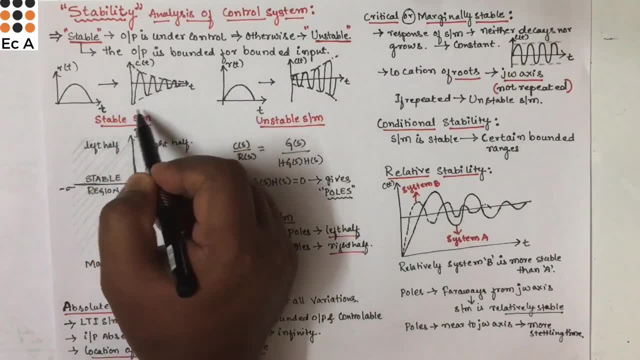 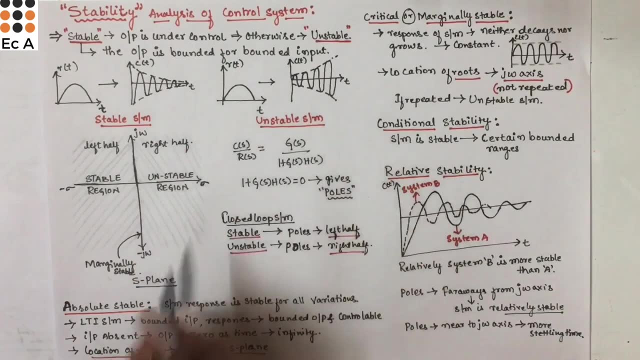 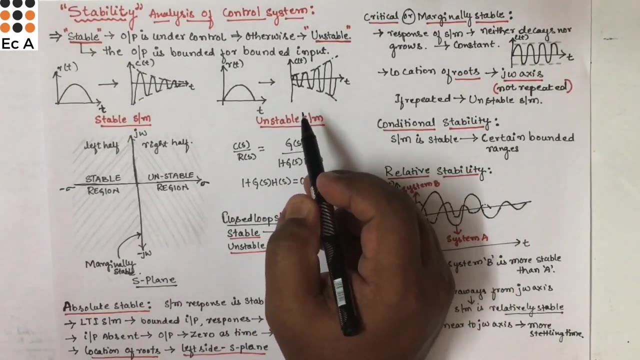 This is the input to the system and this is the response to the system. Here the transient response vanishes as time approaches to infinity. Such type of system are known as stable system. If a system is unstable, if the output of the system is unbounded for any bounded input, 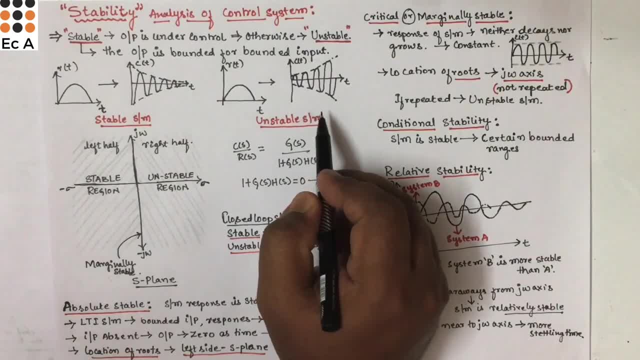 So for a bounded input. if we get unbounded output, we will call such type of system as unstable system, stable system So, which means once the input is given, the output of the system goes on increasing and the user does not have any control on the output of the system. Such type of system is: 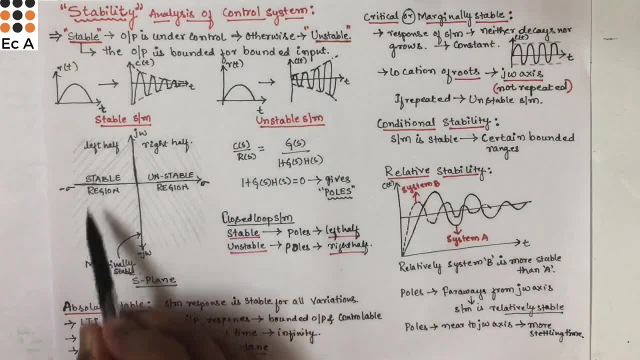 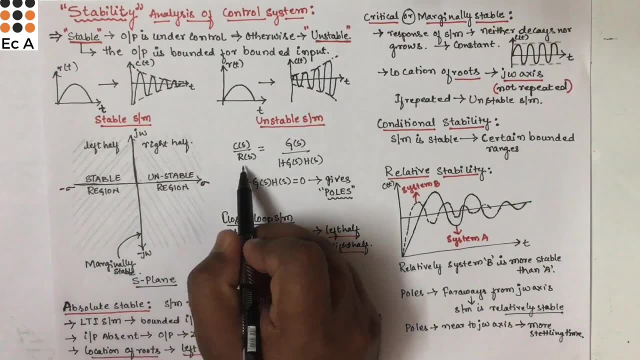 known as unstable system. This figure shows the S plane and the location of stable region and unstable region of the system. If we consider the transfer characteristics of a closed loop system, we can write that as G of S divided by 1, plus G of S into H of S. If we take the 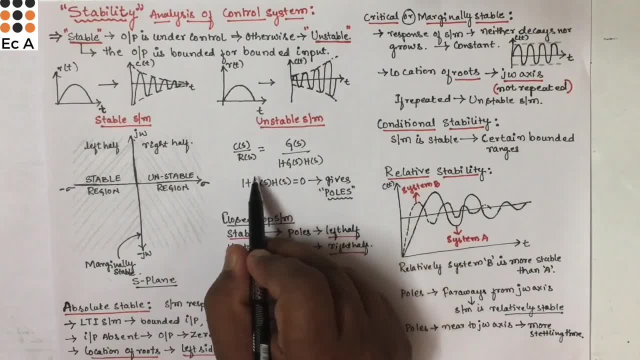 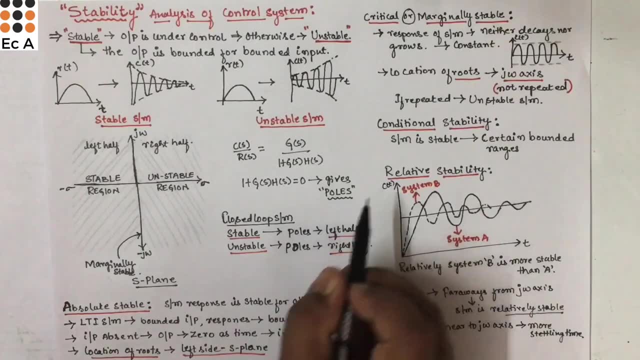 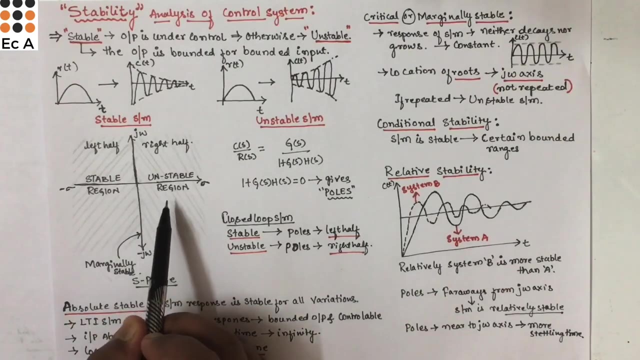 denominator and equate that to 0, we will get the equation which is known as characteristics equation. From this characteristics equation we can find the poles, and the location of the poles in S plane will decide whether the system is stable system or a unstable system. In a 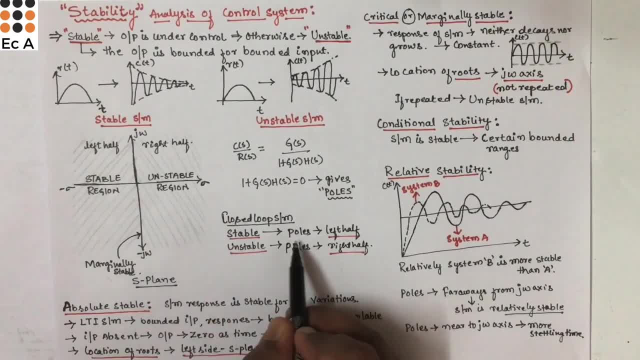 closed loop system. a system is said to be stable if the poles are located. I will write that as G of S divided by 1, plus G of S into H of S, If we take the denominator at the left half of the S plane. if the poles are located at the left half of the S plane, 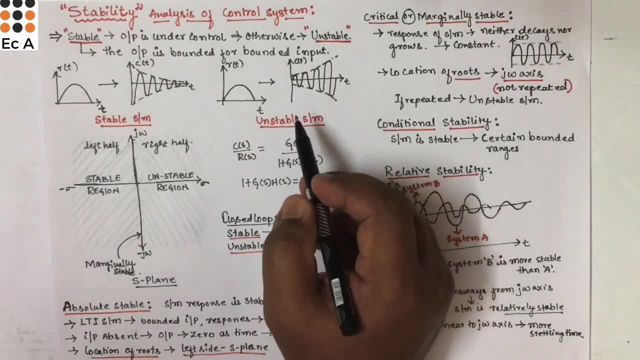 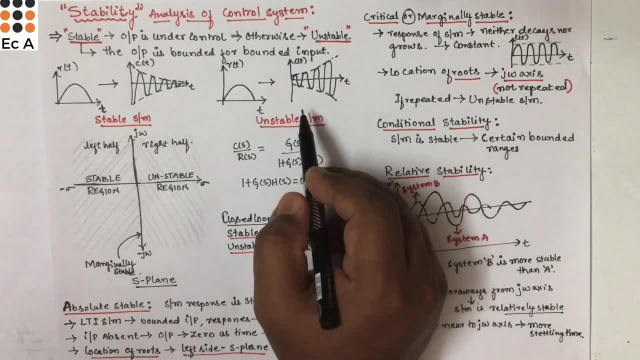 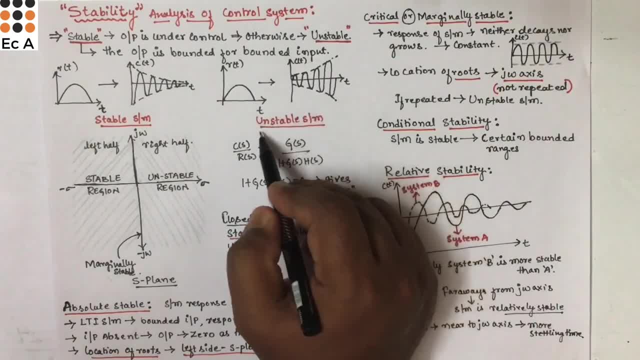 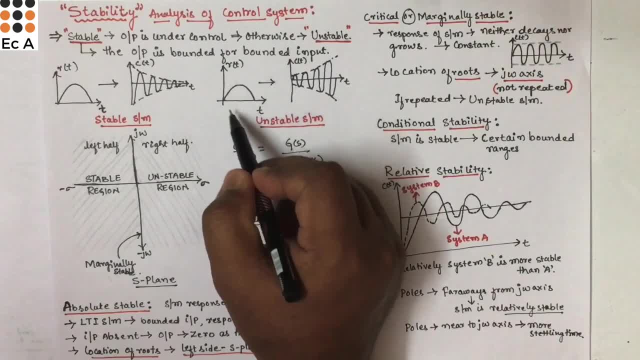 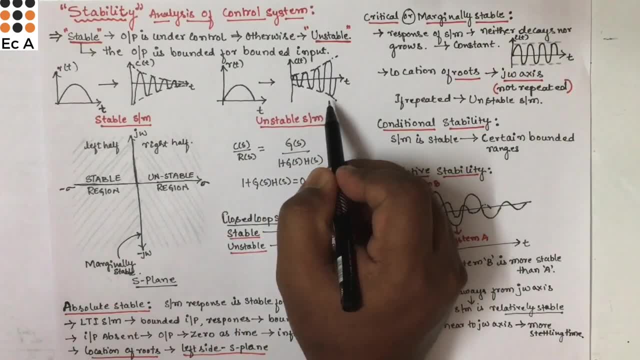 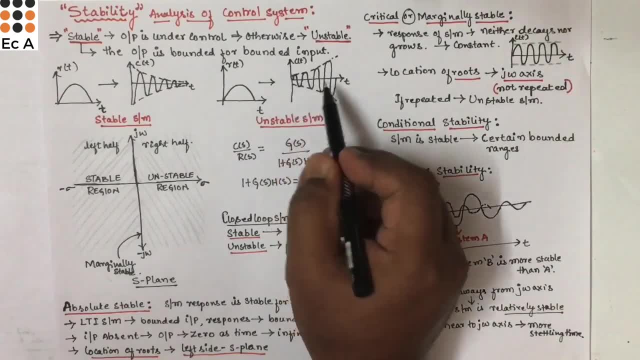 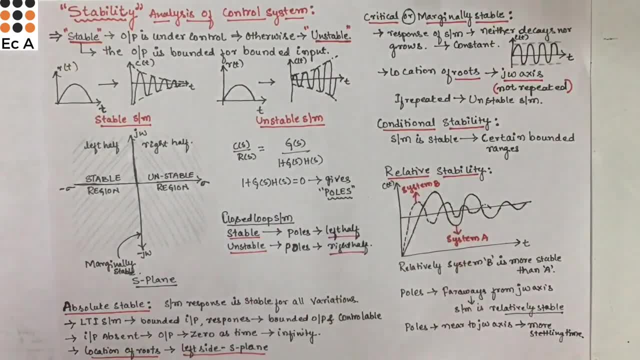 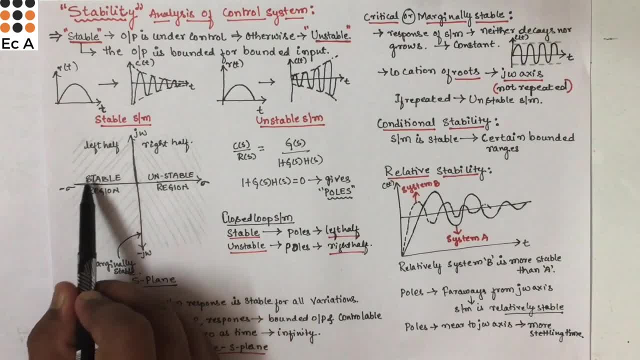 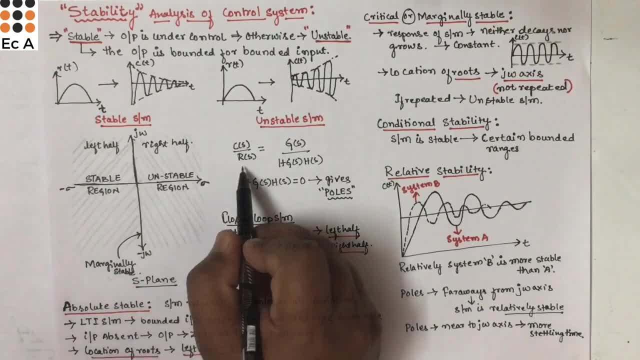 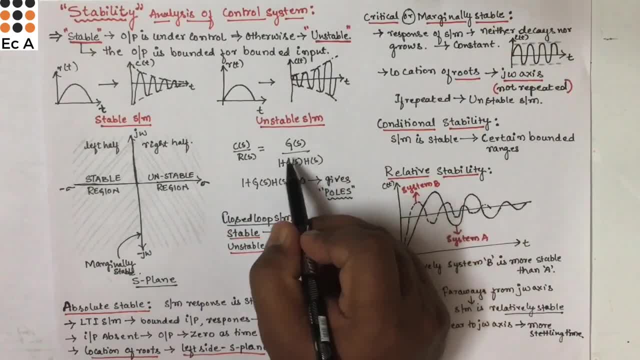 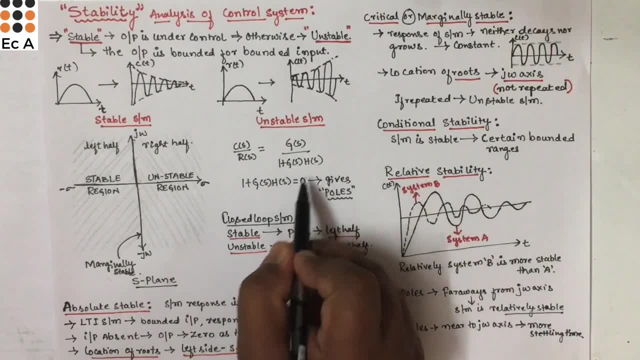 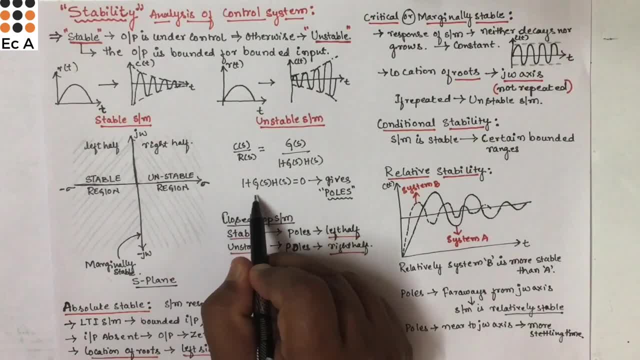 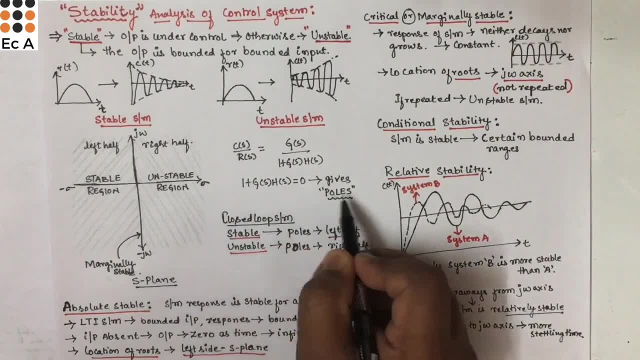 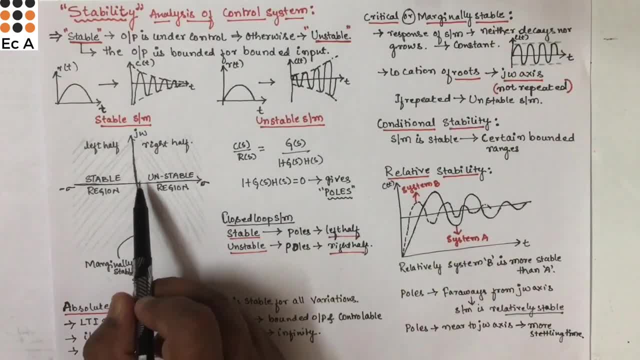 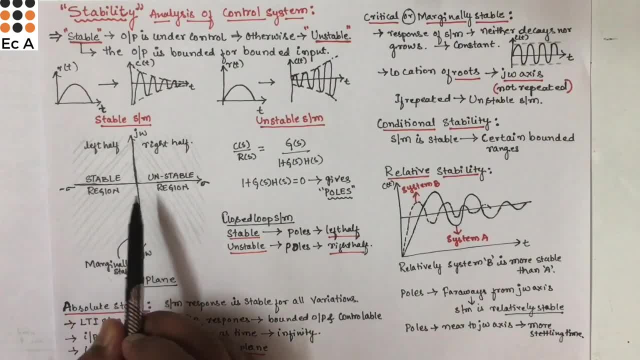 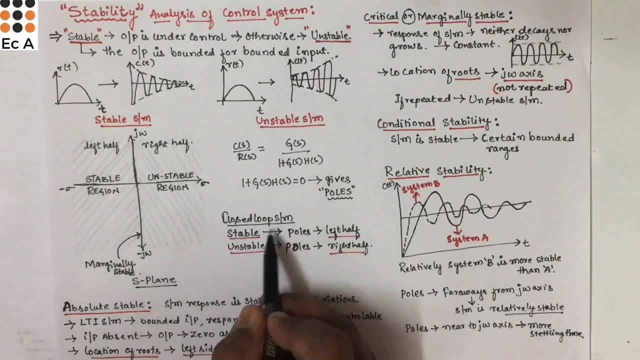 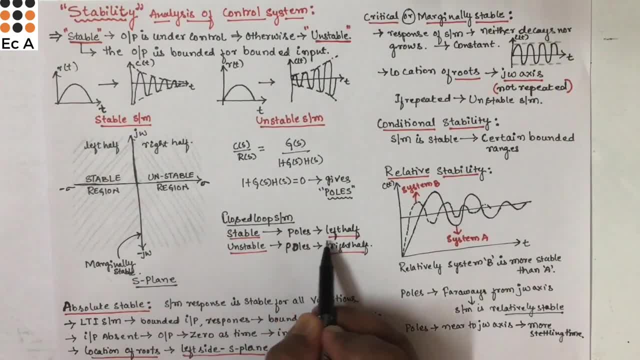 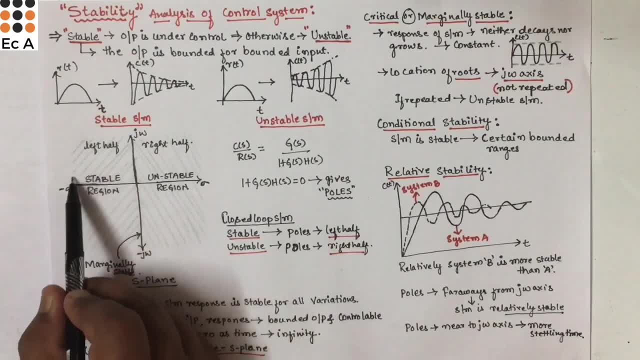 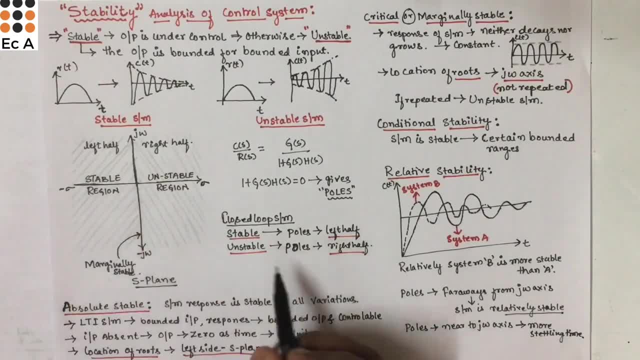 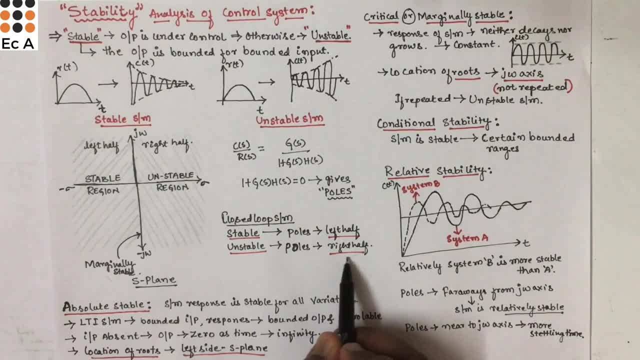 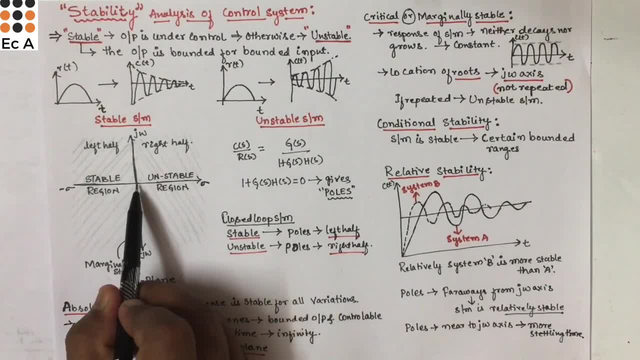 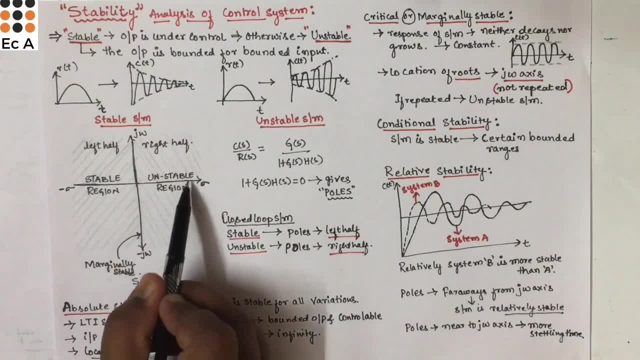 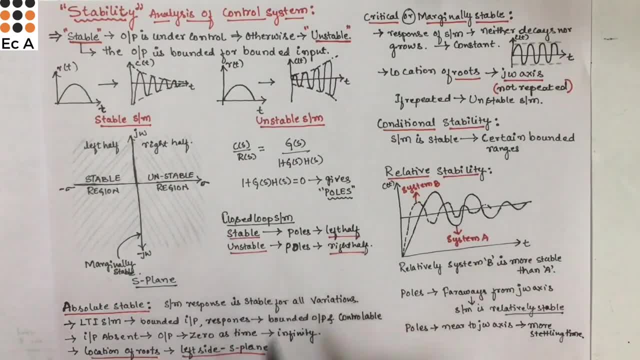 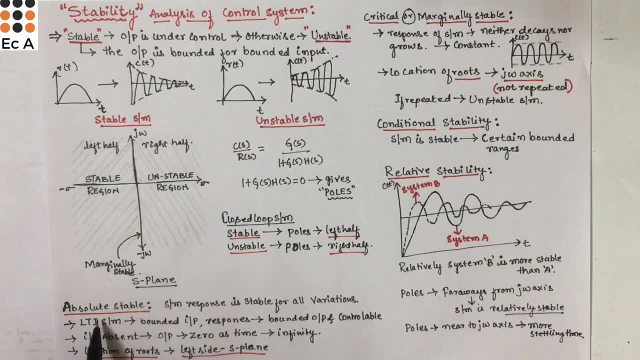 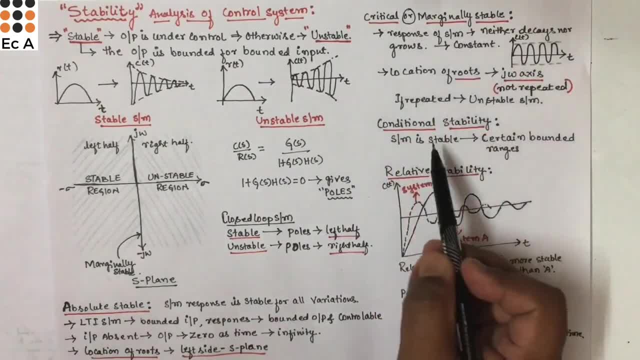 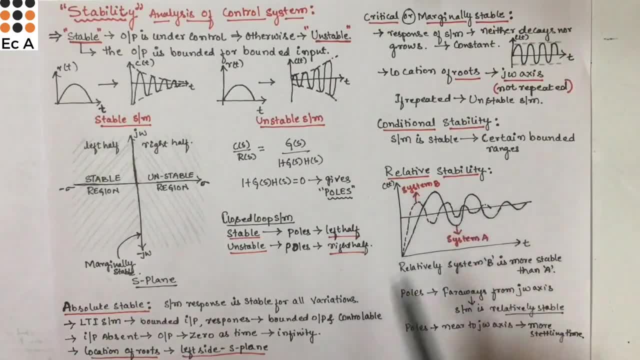 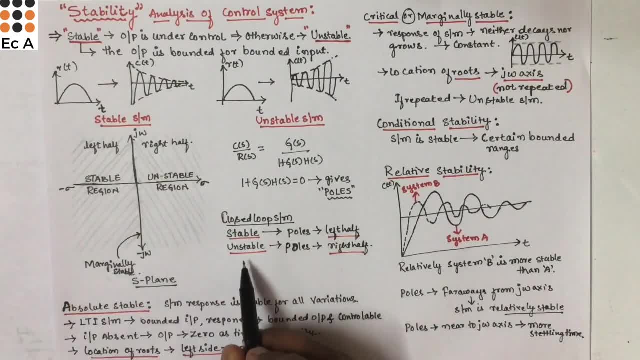 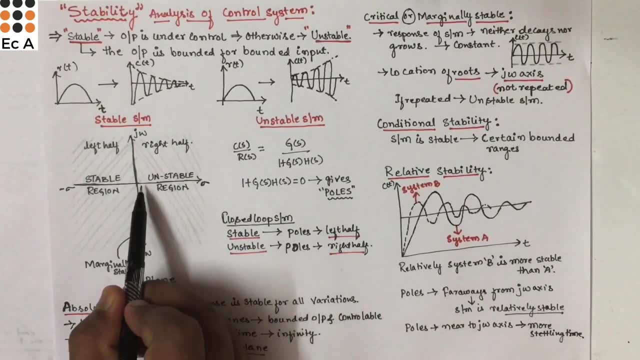 we call such type of system as stable system. If the poles of the system is located at the right half of the system, we will call such type of system as unstable system. So in the S plane, if the poles are located at the right half, we will call such type of system, as known as unstable. 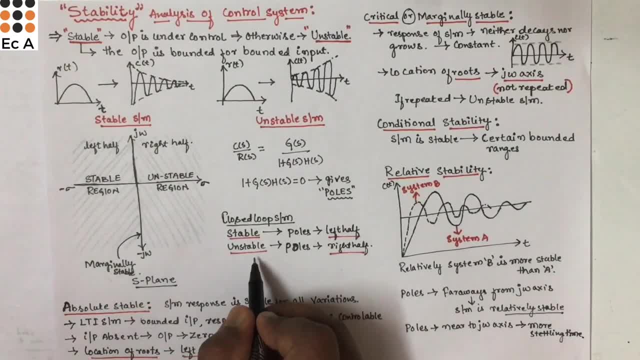 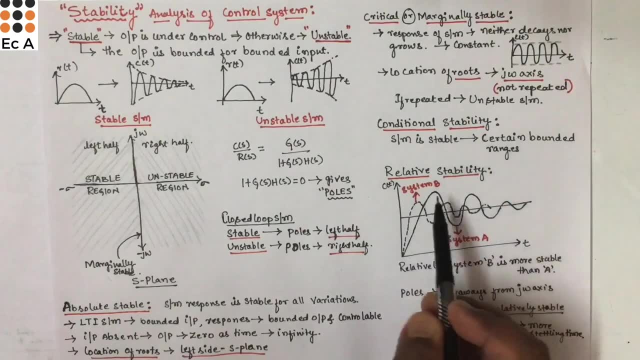 system, Along with stable system and unstable system. we are having absolutely stable system, critically and marginally stable system, conditional stability as well as relative stability. first let us understand what is absolute stable system. a system is said to be absolute stable if the system response is stable. 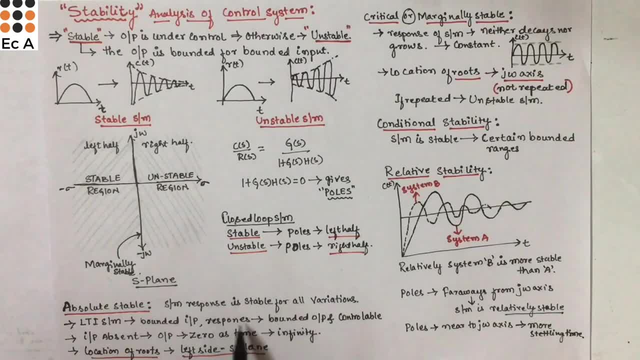 for all variations. if the system response is stable for all type of variations, such type of systems are known as absolute stable system. if we consider an LTI system for a bounded input, the output should be bounded as well as controllable. if the output is bounded for a bounded input and if we 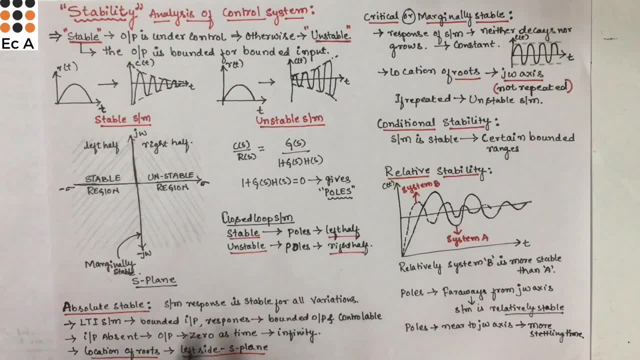 can control the response of the system. such type of systems are known as absolute stable system. in this type of system, if input is absent, at that case the output should move to 0, or the output should approach 0 as time approaches infinity. Such type of system is known as absolute stable system. 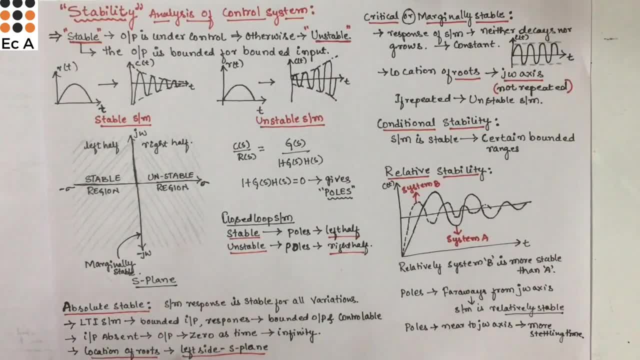 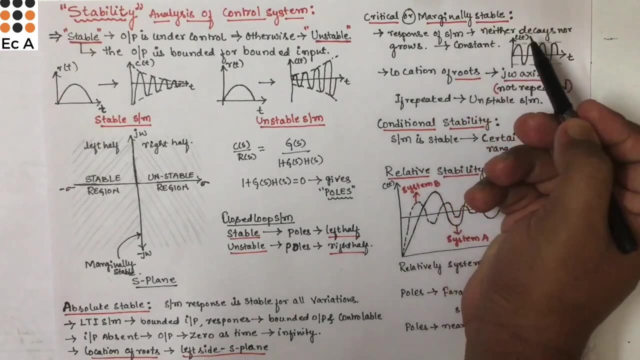 Next type of systems are known as absolute stable system. For this type of system, the location of roots will be on the left side of S plane. If you consider the S plane, the roots will be at the left side of S plane. Next we will understand critically or marginally stable system. 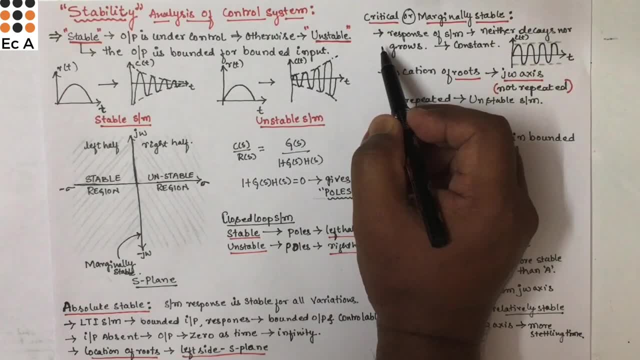 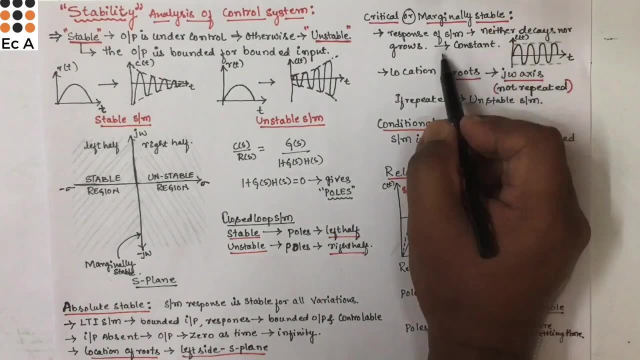 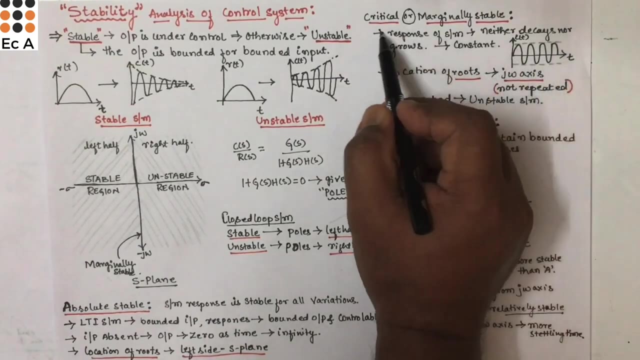 A system is said to be critically or marginally stable. if the response of the system neither decays nor grows, It should remain constant. The response of the system should remain constant. It should not increase nor decrease. Such type of system are known as critically or marginally stable. 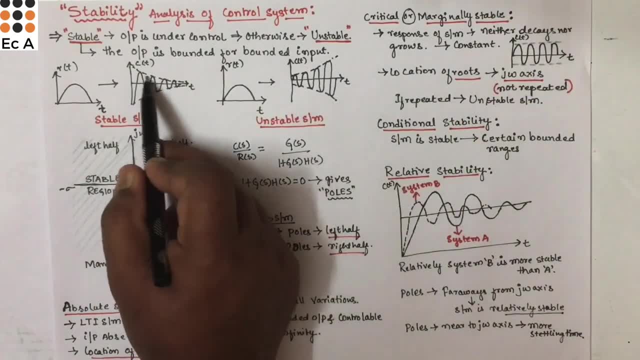 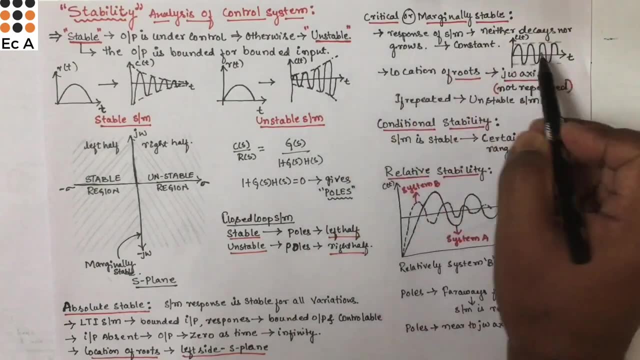 If you can see these two examples, here the response of the system is decaying and here the response of the system is increasing. So in a marginally stable or critically stable system, the response of the system will remain constant. It will neither decay or it will not grow. 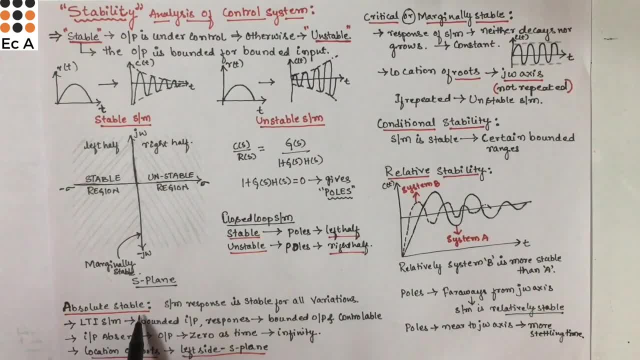 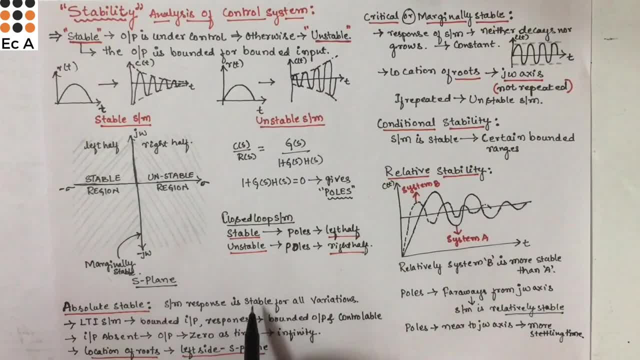 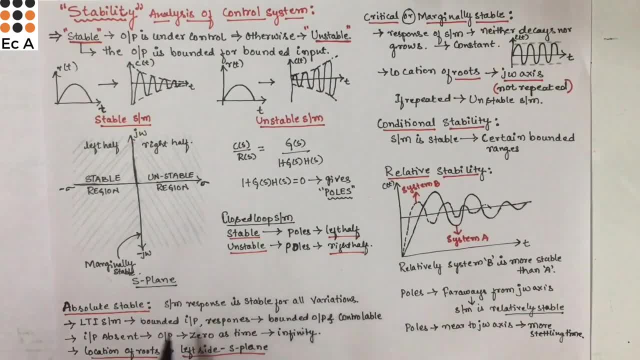 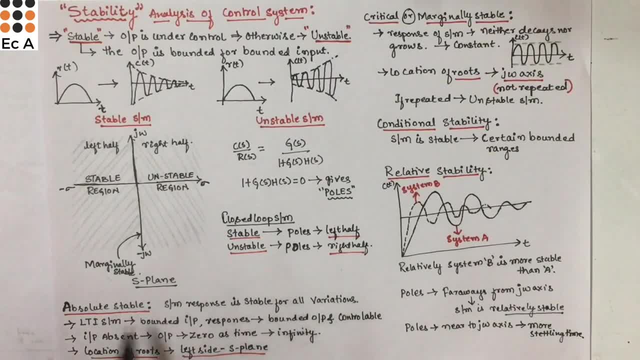 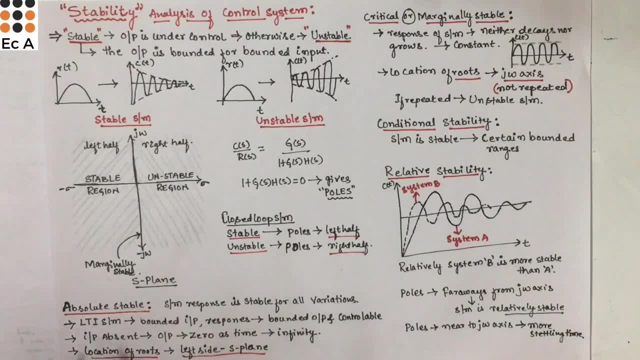 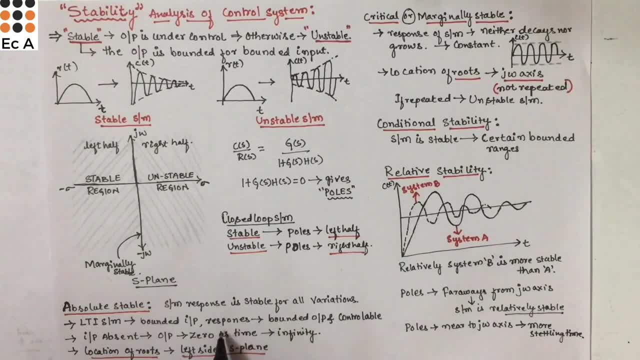 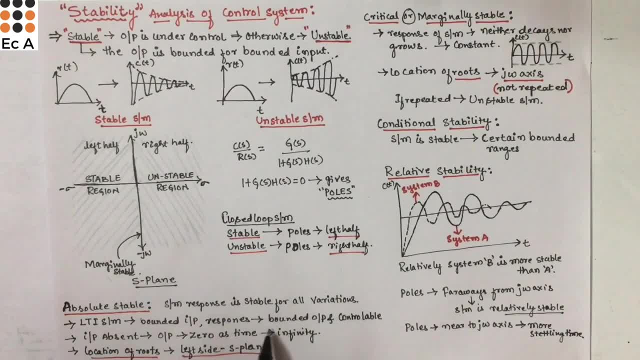 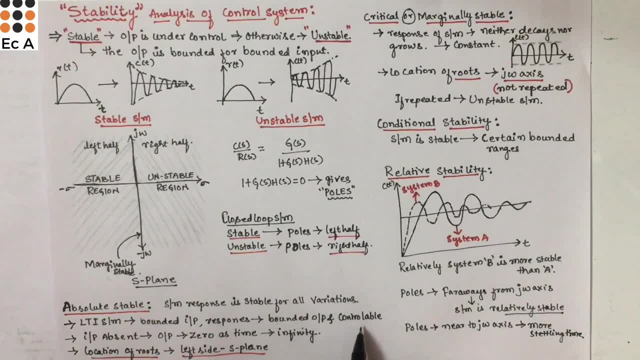 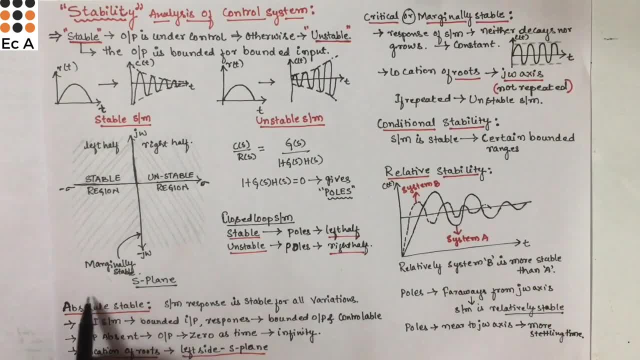 of the system. such type of systems are known as absolute stable system. in this type of system, if input is absent, at that case the output should move to zero, or the output should approach zero as time approaches infinity. such type of systems are known as absolute stable system for this type. 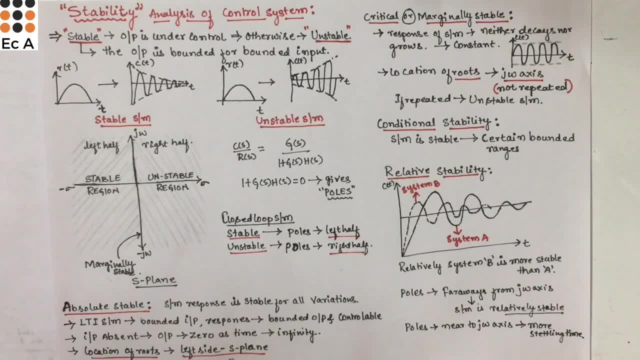 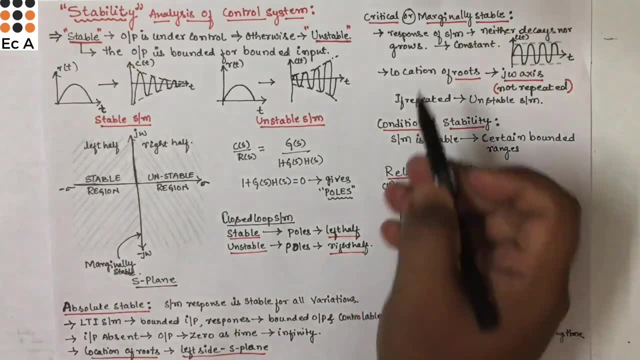 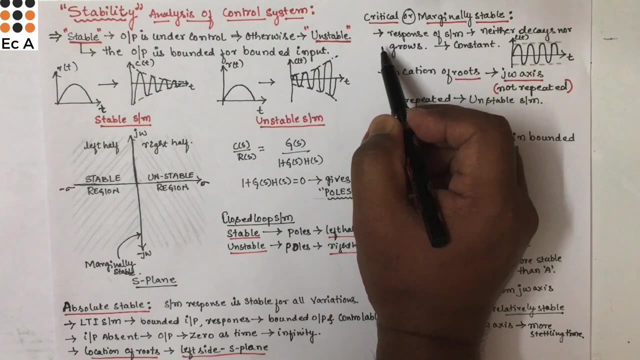 of system, the location of roots will be on the left side of s plane. if you consider the s plane, the roots will be at the left side of s plane. next we will understand critically or marginally stable system. a system is said to be critically or marginally stable if the response of the system 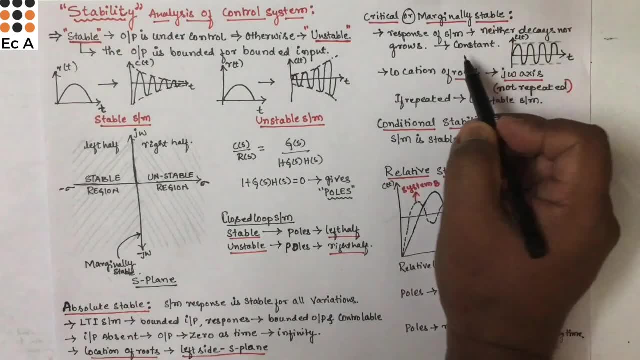 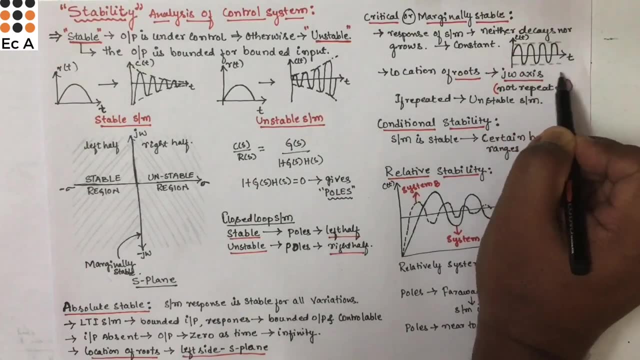 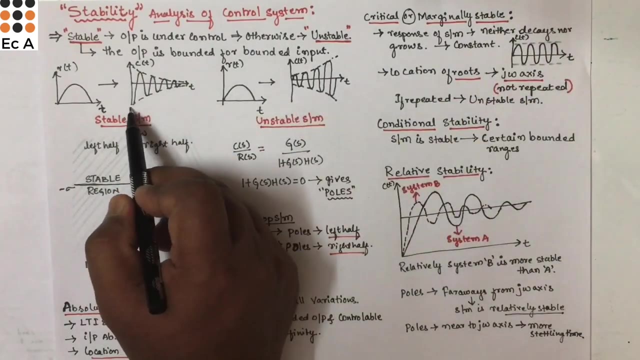 neither decays nor grows. it should remain constant. the response of the system should remain constant. it should not increase nor decrease. such type of system are known as critically or marginally stable. if you can see these two examples: here the response of the system is decaying and here the response of the system is increasing. 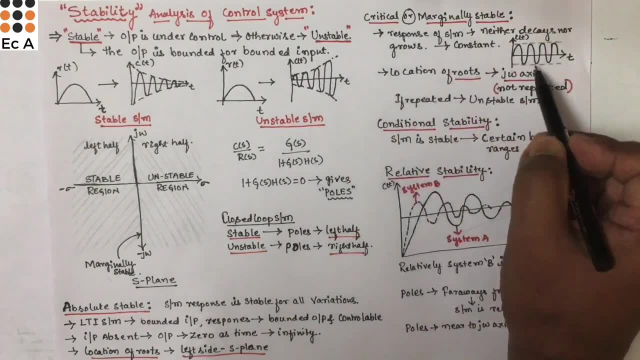 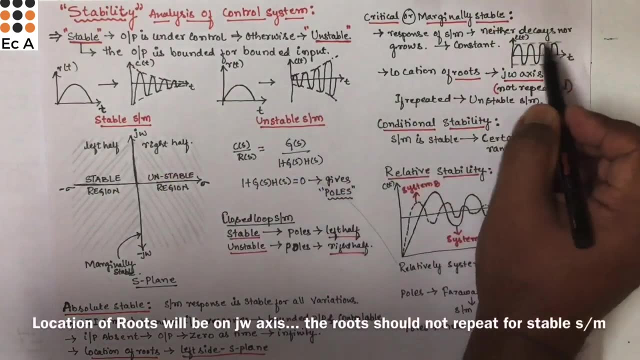 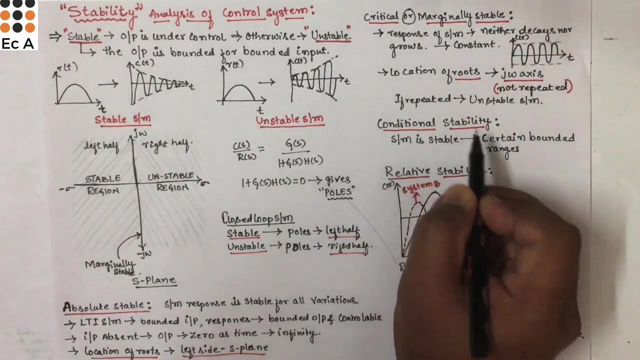 so in a marginally stable or critically stable system, the response of the system will remain constant. it will neither decay or it will not grow. such type of systems are known as critically or marginally stable system. next we will understand conditional stable system. in conditional stable system, the system is stable only for certain bounded range values of 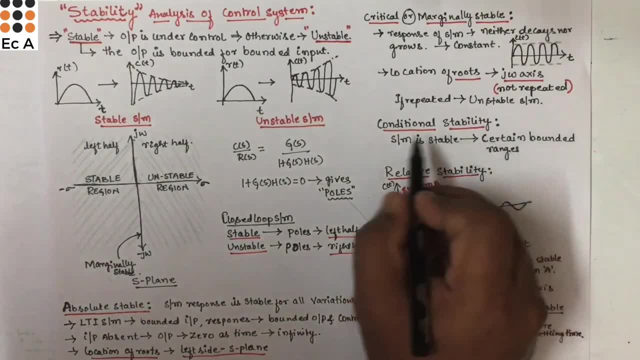 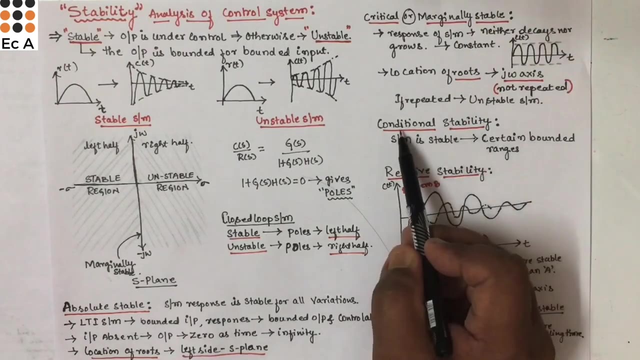 parameters. so only for certain values the system will be stable and for remaining values the system will be unstable. such type of systems we will call that additional stability system. so the system is stable only for certain values of parameters. such type of systems are conditional stable system. next, 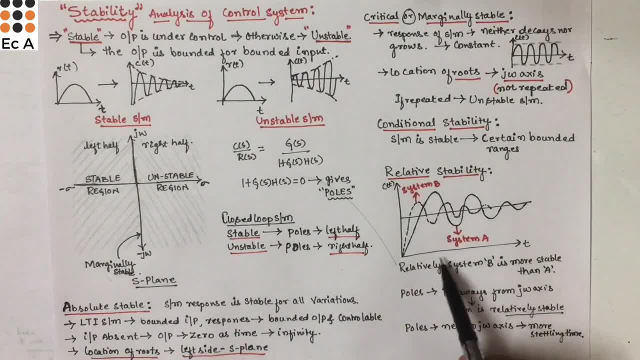 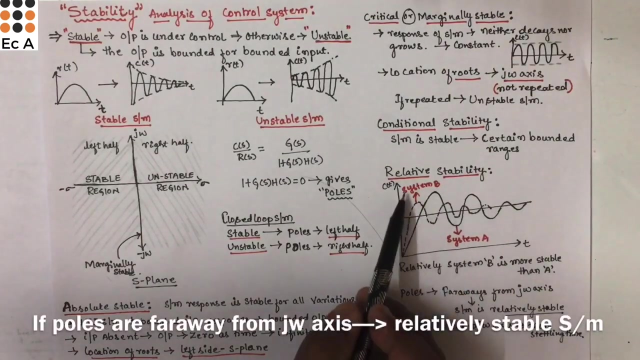 we will see the relative stability. for this, let us consider the response of two systems, system a as well as system b. system a: it is decaying slowly as well as it is taking more settling time, and the response of system b is decaying quickly as well as it is taking less settling time. so, comparatively, or 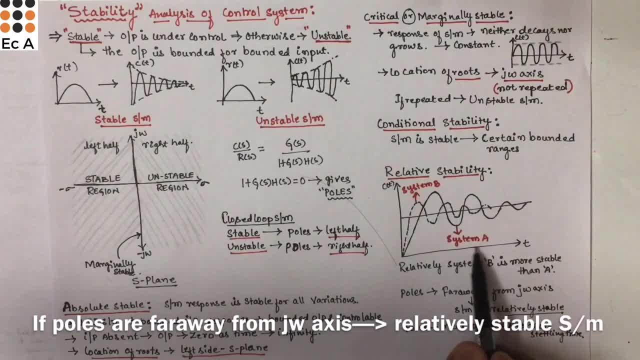 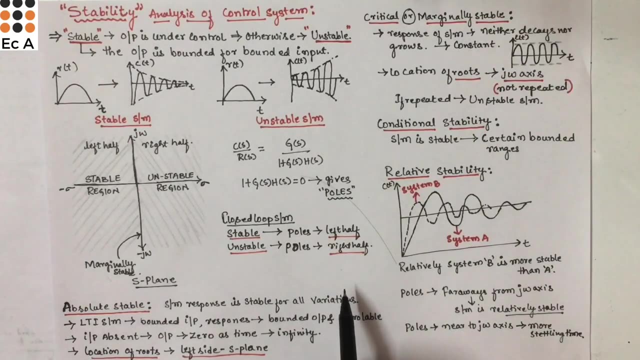 relatively, system b is more stable compared to system a, so such type of system we call that as relative stability system. so this is about the introduction to stability analysis of control system. hope you have understood the topic. thank you.